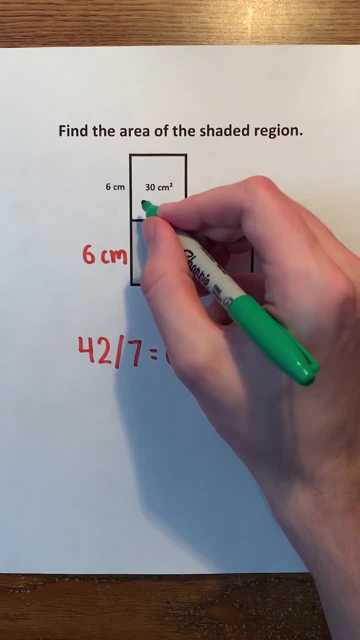 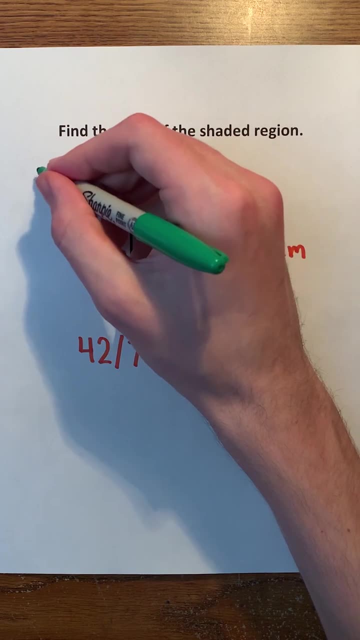 this side, In this other rectangle, we know that the area is 30 centimeters squared and this side of the rectangle has a length of 6 centimeters. So we can divide 30 by 6 to get 5, which means 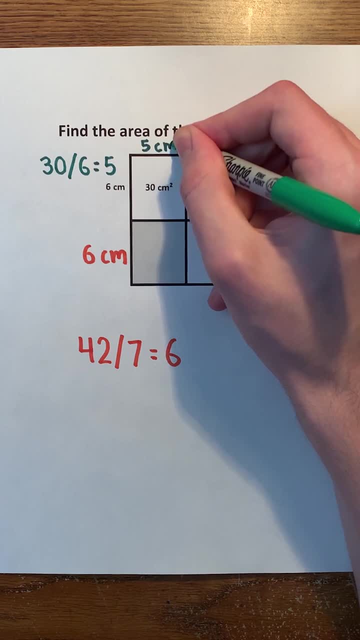 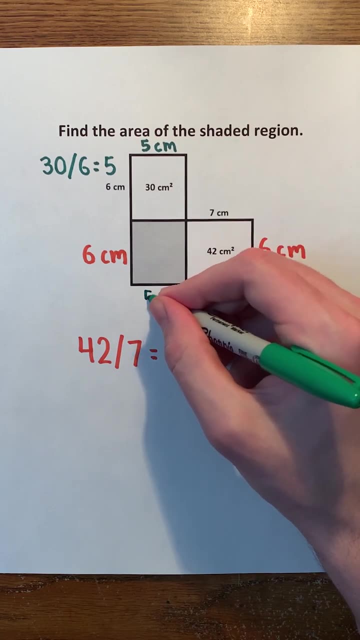 that this side of the rectangle has a length of 5 centimeters. 5 times 6 is 30.. Because this shape is also a rectangle, this side of it must also have a length of 5 centimeters, Because this shaded region is a rectangle and we know the length of this side. 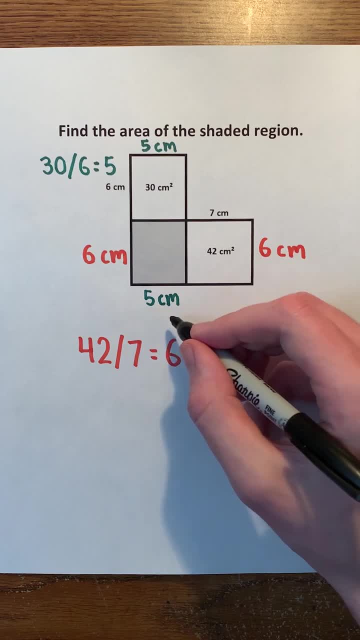 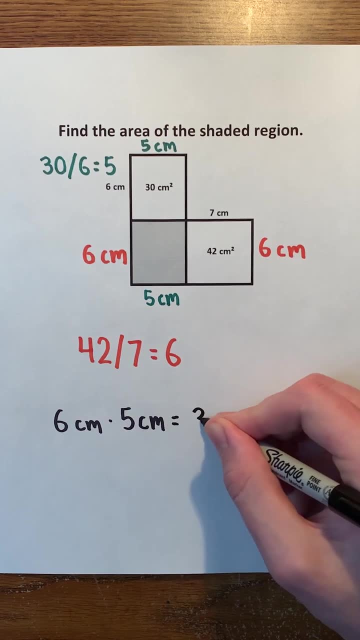 which is 6 centimeters, and the length of this other side, which is 5 centimeters. we can multiply them to find the area of the shaded region. 6 centimeters times 5 centimeters is just 30 centimeters squared. So 30 centimeters squared must be the area of the shaded region. 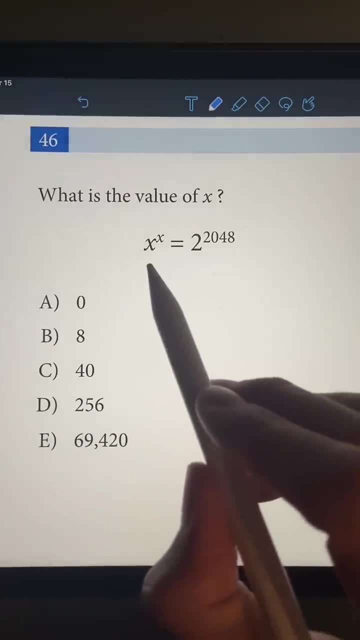 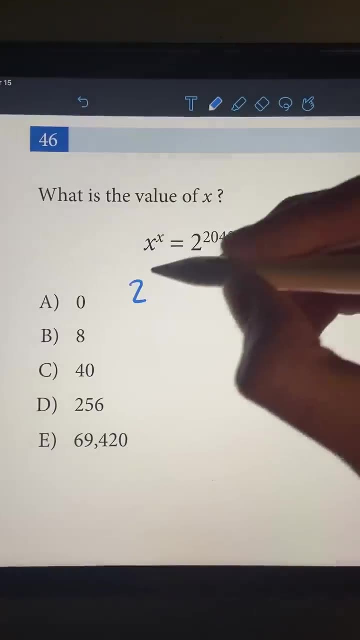 Problem is super weird, but I'll show you how you can solve it. So we have some number to the power of itself is equal to two to the power of 2048.. So the first thing I'm going to do is rewrite this exponent. So I'm going to rewrite it as two to the power of two times 1024.. So what? 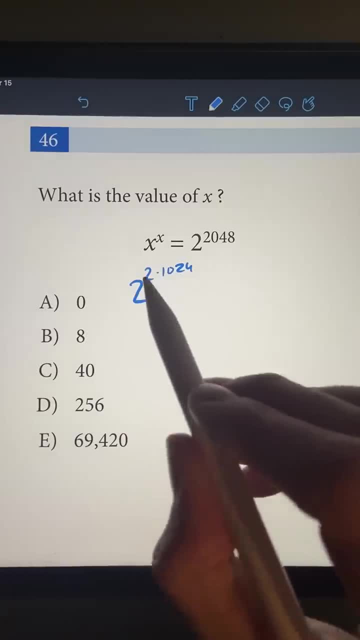 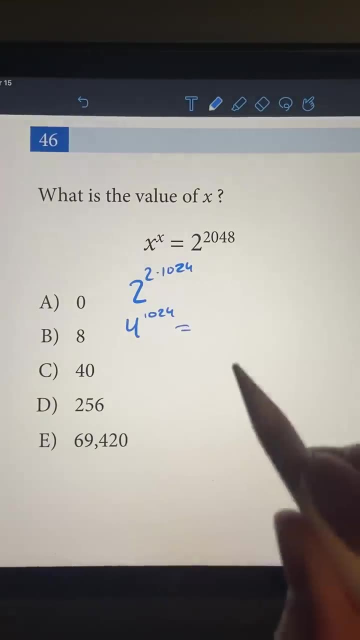 that does, is it? lets us rewrite this as a new base. So two squared is going to be four. So our new base is four. We still have a 1024 as our exponent, So now I'm going to keep repeating this process. So I'm going to rewrite it as four to the power of two times 512.. So our new base is: 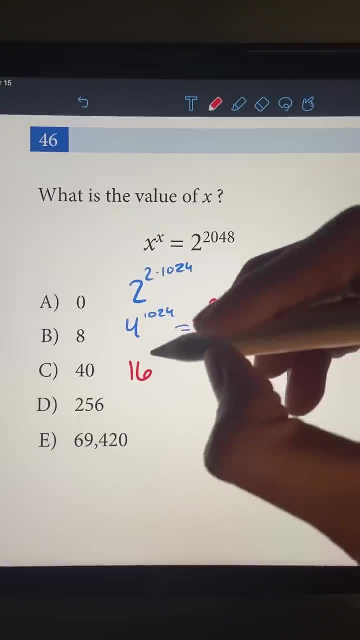 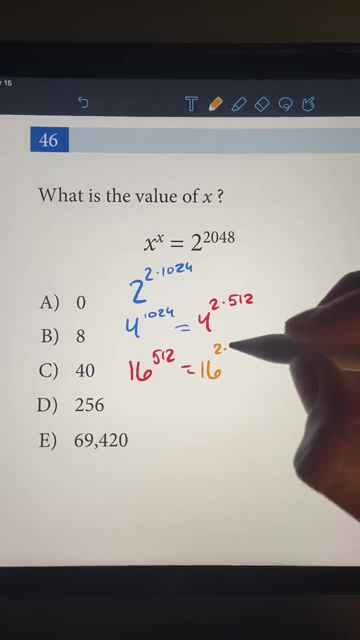 just going to be four squared. So we have 16 to the power of 512.. So let's do this one more time. So we have 16 to the power of two times 256.. So our new base is 16 squared, which is just going. 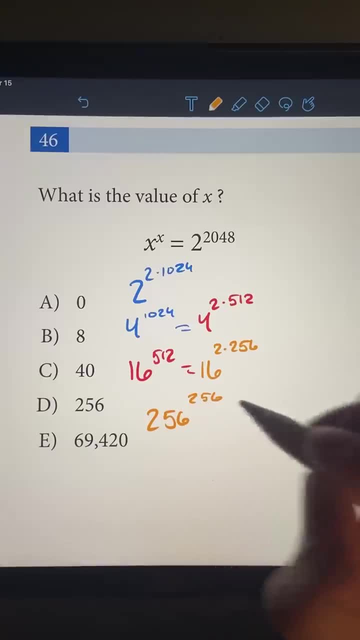 to be 256. And we have a 256 as our exponent And just like that, we found a number to the power of itself, which is 152.. So we have 16 to the power of two times 256. So we have 16 to the power of. 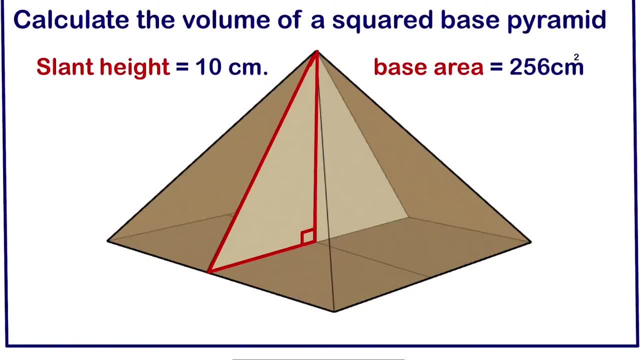 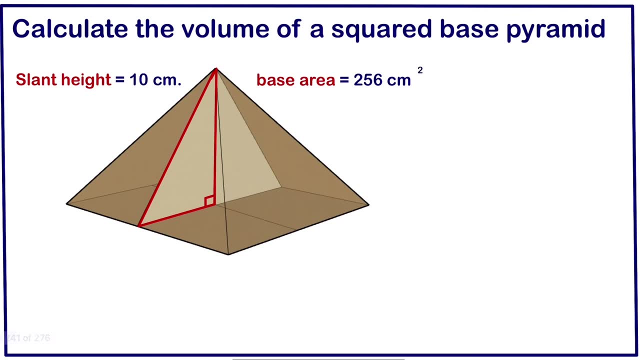 Welcome to Mathematics Pro. So today we are going to calculate the volume of a square base pyramid. So they gave us the slant height and the base area, So let's get started. So we are asked to calculate the volume. So the first thing to do is to write the formula of volume so that we should know what is needed for us to calculate the volume.